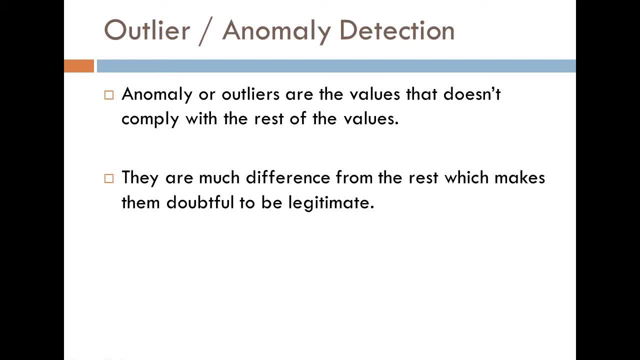 from being part of any cluster. Other than that, every technique was accommodating outliers to be part of the cluster and due to that, the original shape of the cluster was tempered. So what actually outliers are? Outliers can also be called anomalies, and these are the 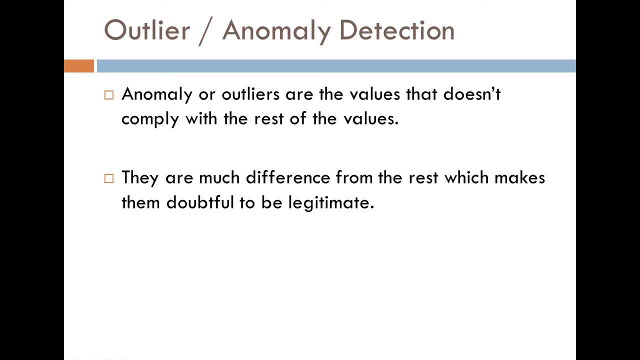 points or the objects or instances or documents that do not have any outliers, They are actually not compliant with the rest of the values. So if we have got a dataset and in that dataset we have different users and their buying patterns, If there is a user whose buying pattern is very much different from the rest of the data, 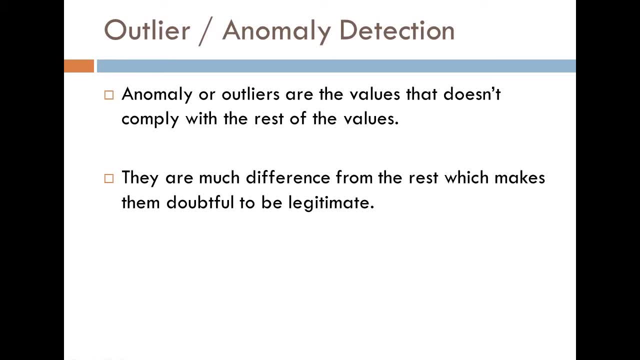 so that is most probably an outlier. And generally, how outliers can be identified are that there aren't going to be many values around the ones that are outliers. Its values are going to be a lot more different from the rest of the values If you do not preprocess them. most of the techniques do not know how to deal with anomalies. 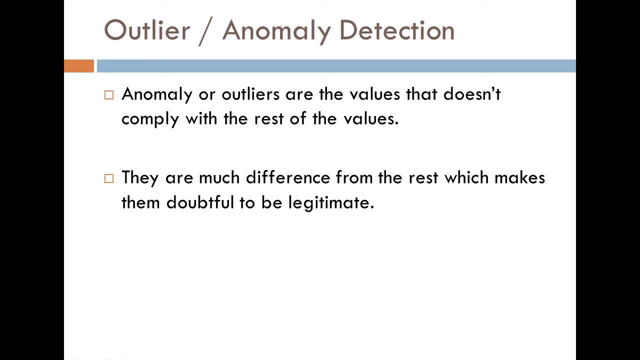 and they are going to affect the results of whatever the classification or clustering techniques that we are using, Others that may deal with outliers would still have problems with correctly identifying these outliers. Therefore, outlier detection and removal is part of preprocessing. In preprocessing we try to get rid of most of the problems, if not all, that we have in 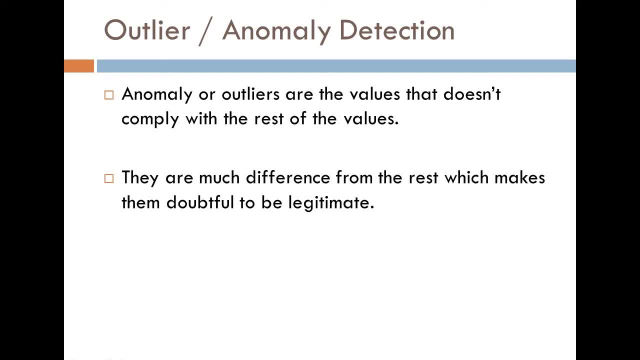 our data so that when we provide that data to the model, it should be trained well. So the objective of preprocessing is to rectify all the problems that we have in our data. This may include noise removal, missing values detection, outliers detection and removal. 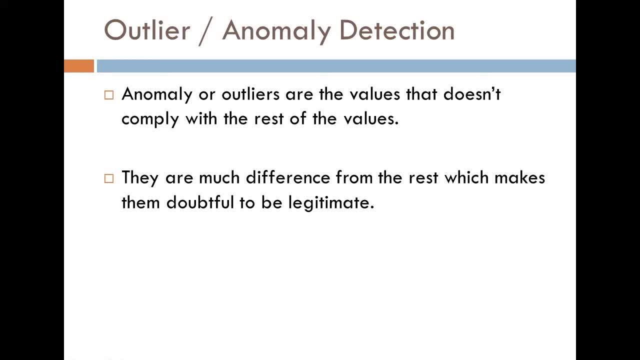 normalization of values to a specific scheme, fixing categorical data and all other such problems So outliers. since they are very much different from the rest of the values, it makes their position doubtful to be legitimate. Either someone mistakenly have added those points and the values are not accurate, or the behavior of that person is so unlike the rest of the.